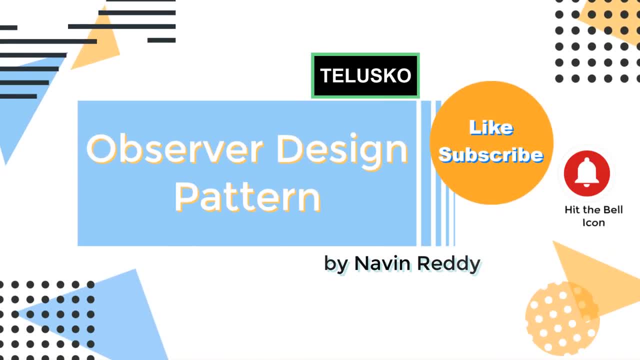 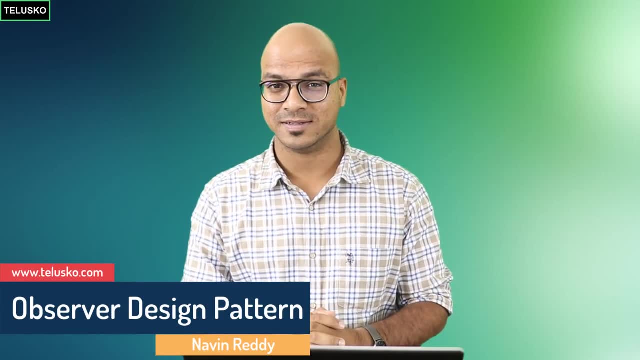 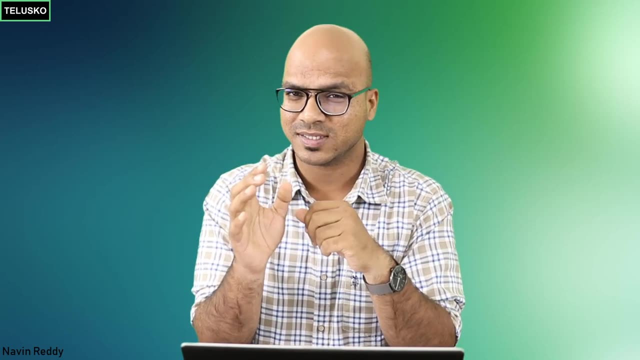 Welcome back, Aliens. my name is Devyn Reddy and in this video we will talk about observer design pattern. So we had some design pattern videos before and now it's time for observer. But why do we need it? To understand this concept, let's take an example of YouTube. 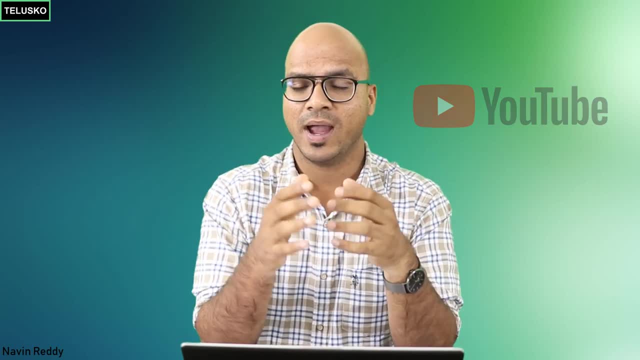 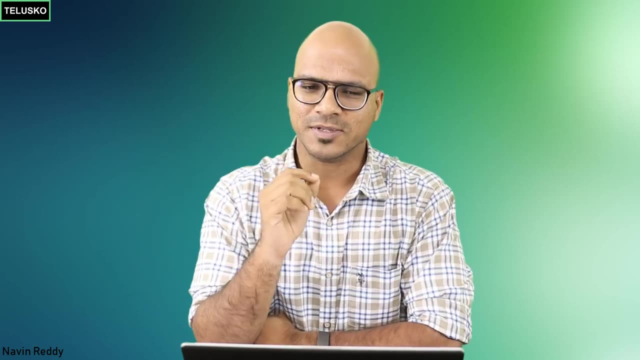 So on YouTube, we have so many channels, right- One of them is Tedisco- and then we have so many subscribers- In fact, we have a lot of viewers- and then some of them subscribe the channel, So they become a subscriber. Now what happens is, every time I upload a video, 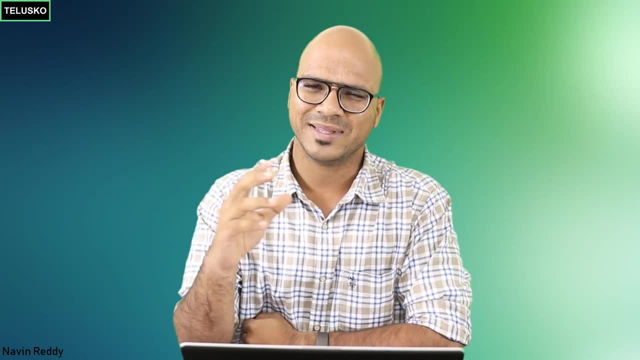 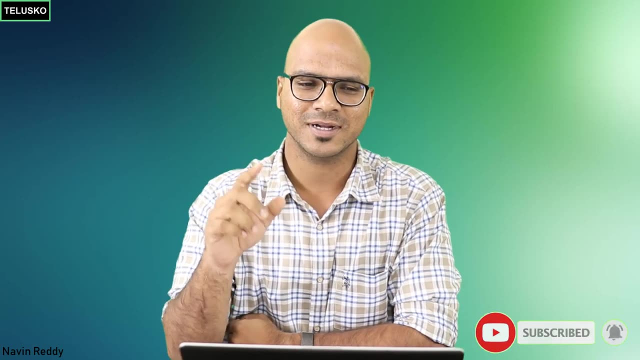 you will get notification, and that's the importance of subscribing the channel. But now we also have a bell button there, but that's a different thing. I hope you have clicked on that subscribe button and then hit that bell icon. That's very important. So every time we upload a 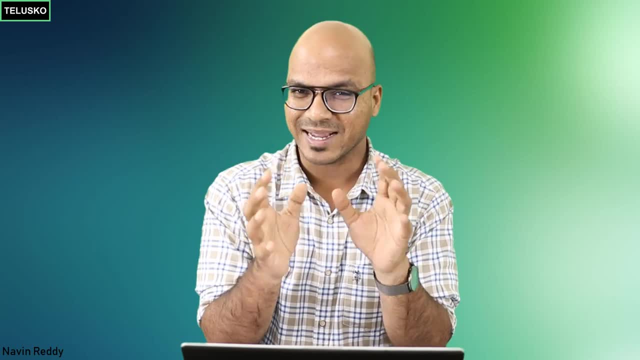 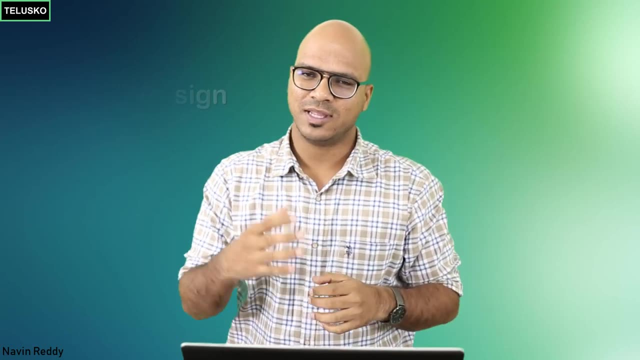 video. you will get a notification that there's a video uploaded. That's how the YouTube works. right Now. they have implemented the observer design pattern. Okay, so let's imagine. let's say: if you want to build this concept, you know, if you want to. 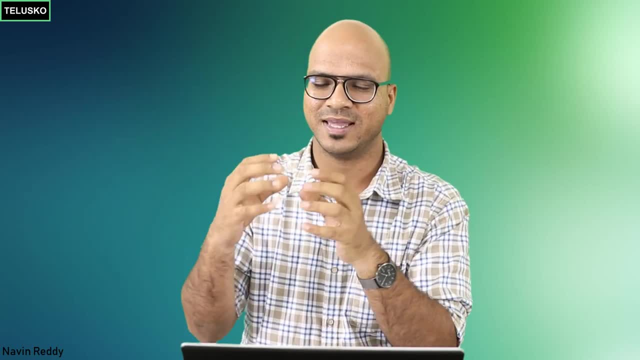 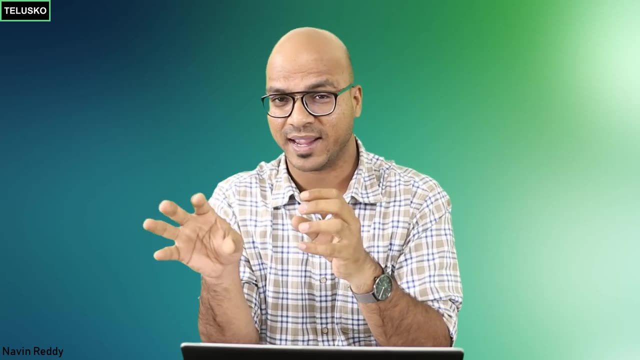 build this programming. So let's say we have a YouTube object, a big YouTube object, and then inside that you'll be having channels, right, And then you will be having subscribers. Both are two different entities here, So we have channel and we have subscriber. Now 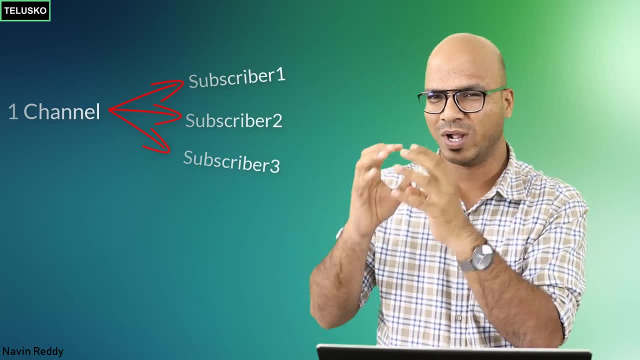 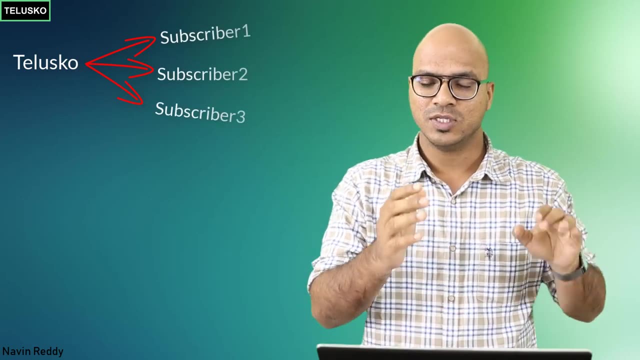 of course, one channel will have multiple subscribers. So let's only focus on one channel now, Let's not focus on multiple channels. Let's say, on YouTube we have only one channel, Tedisco, and then we have so many subscribers here, So it's more about one to many. So we 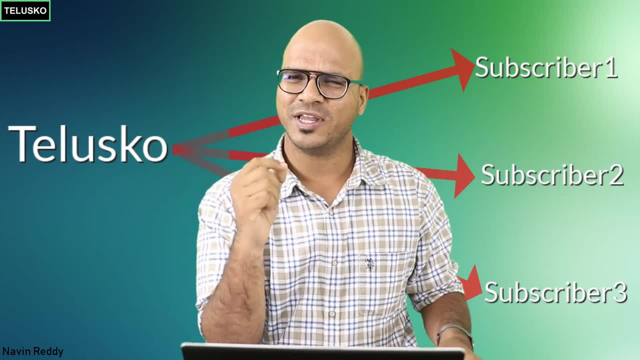 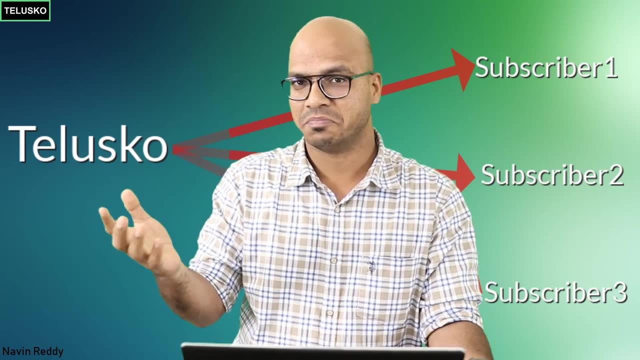 have one channel and multiple subscribers, right? So let's say you're waiting for a video on this channel. Okay, so what? you will do so every morning you will. at 9am you will check. Hey, do we have a new video from Tedisco? No, it's not there. You will again check at 6pm, Is it there? 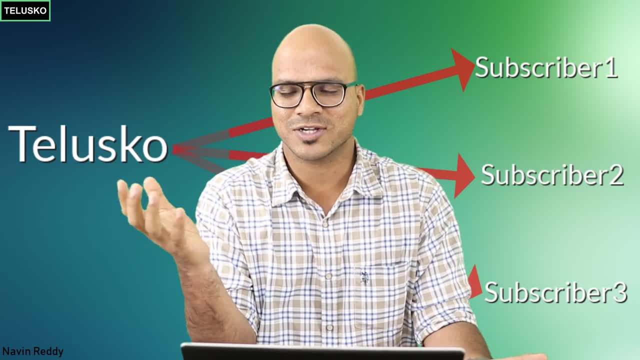 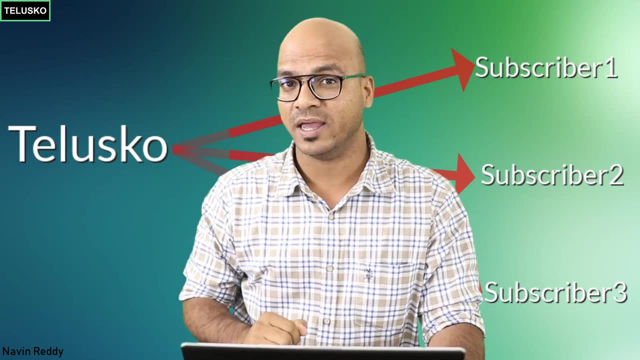 It's not there. I hope people will wait like this. But yeah, that's how things work, So you have to wait. you have to go to channel every time to check for new updates Now, instead of subscriber going to the channel to verify what. if the moment you upload a video, the 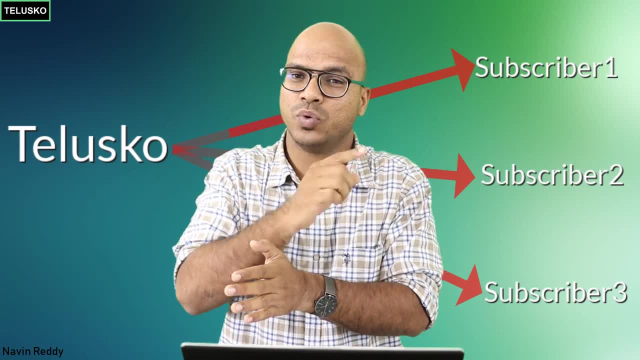 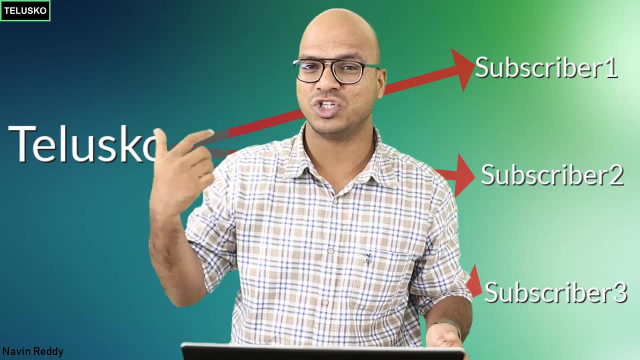 moment I upload a video, the channel will send a notification to everyone. So which is better? Is it the pull request or the push? Now, what is pull basically? So you're going to channel to check if I have a new video that's pulling, because you're pulling the. 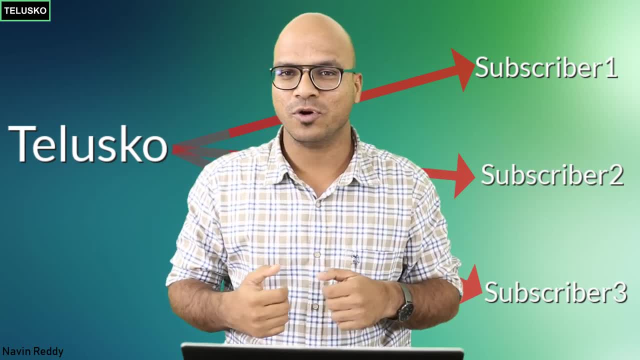 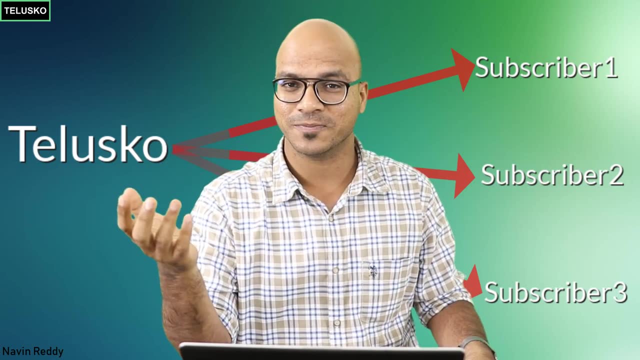 pulling the information. On the other hand, I can push. you don't have to pull for that, right. So you will be saying: okay, whenever Tedisco upload a new video, you will get notification. So you don't have to worry about when I'm going to upload a new video, right? So what? 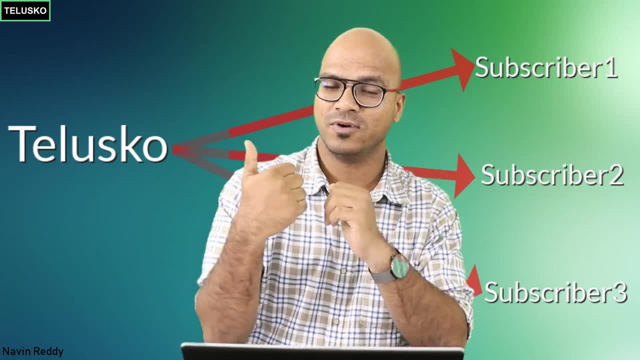 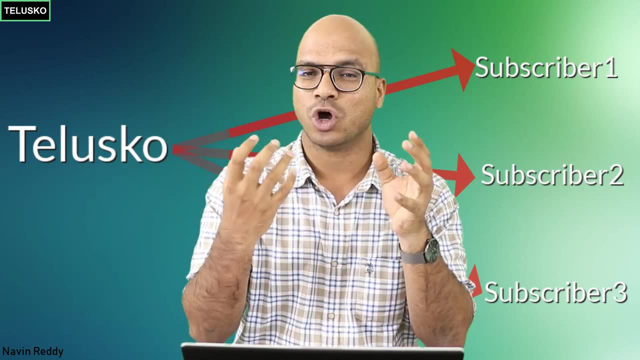 you're doing is you have basically said: Hey, I want to observe Tedisco. The moment you say you are observing it, every time I upload a new video, you will get the notification right. That is observer design pattern. So basically, that's what you're doing, right. So you're. 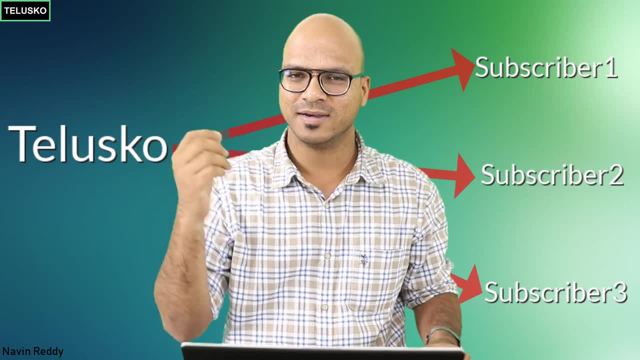 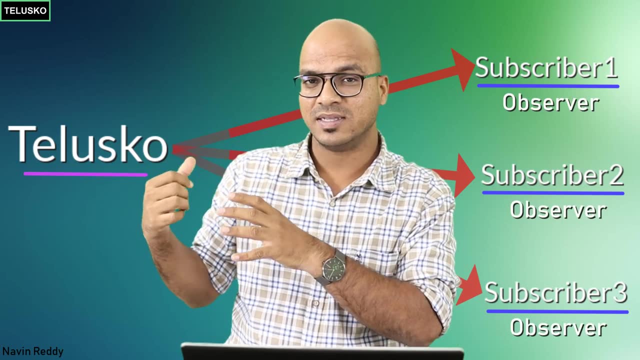 going to channel to check if I have a new video right. So what you're doing is you have. basically, we have a lot of subscribers, we have a channel here and you will be observing. So you can say the. the subscribers are observers And the channel is a subject, because, as an observer, 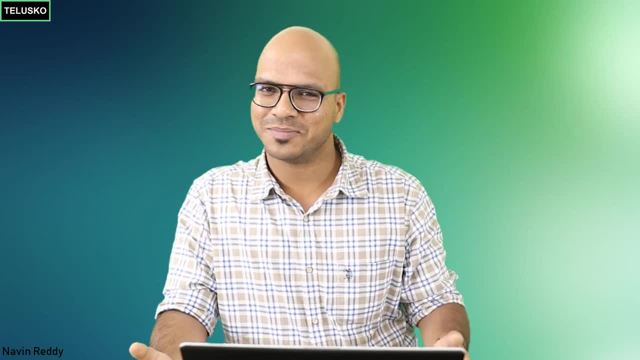 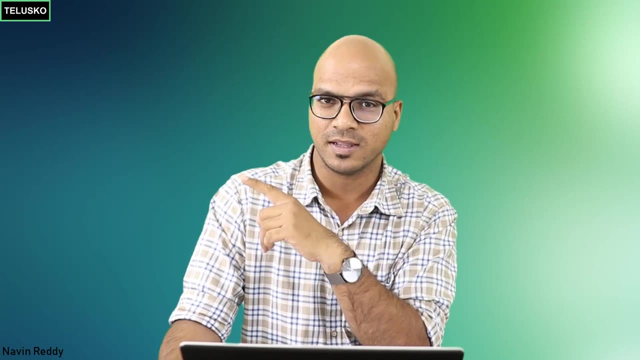 we observe a subject, right? Let's say, if you go to a museum, you observe a subject. So that's, that's what observer design pattern is It's all about? you will first subscribe the channel And then, every time a channel update uploads a new video, you will get notification. 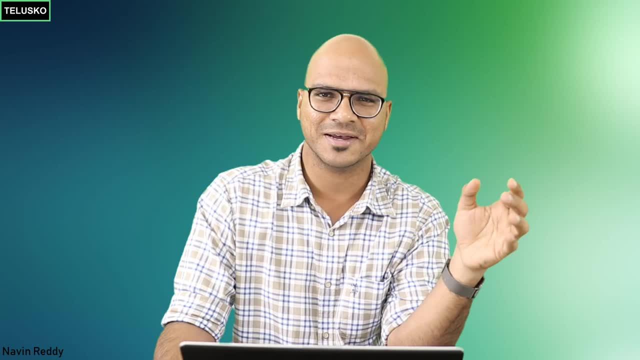 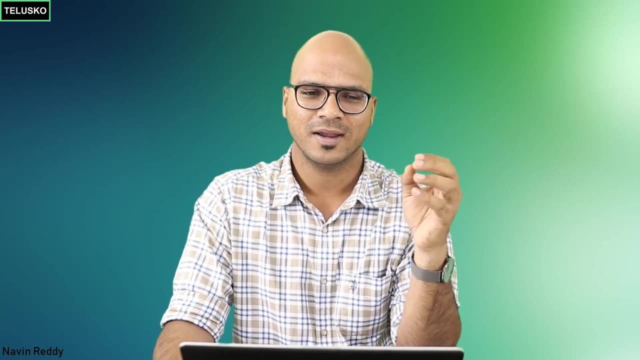 Okay, instead of saying channel will say subject. instead of saying subscribers will say channel will say observers. right, So those are technical terms with which they use in books. But again, different books have different conventions. So in this code we are going to focus on 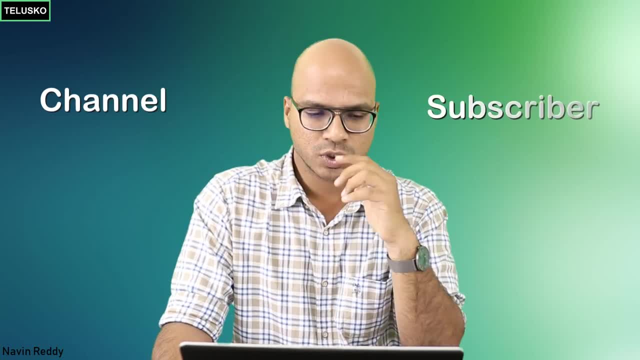 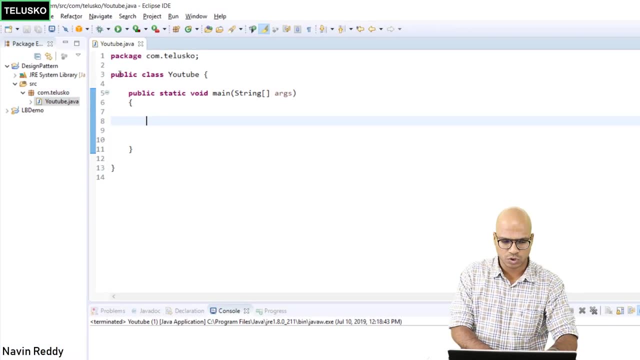 this keyword, which is channel and subscriber. So what I want to do is I want to build something like YouTube, where every time I upload a video, you will get notification. Now to achieve that, let's go to the code And here let me create a class, and this will start with subscriber. 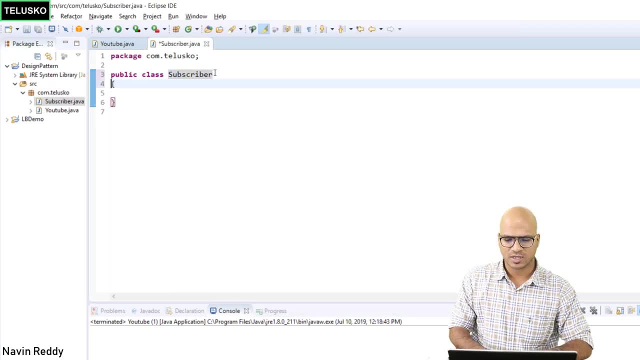 first. So let's get a class which is subscriber. Now, when you say you're a subscriber, of course you will be having certain properties right Now, one of the property- very important- which is private string name. So of course every 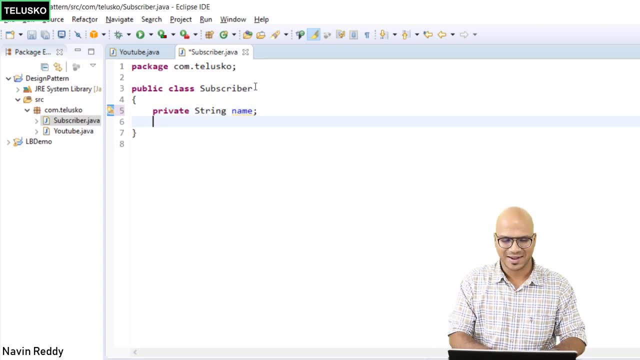 subscribers has a name And it can be a fake name, that's fine, But you will be having a name. And the second thing is you have to also mention to which channel you have subscribed. So we'll say private channel, channel, right, So as a subscriber, when you say you're a 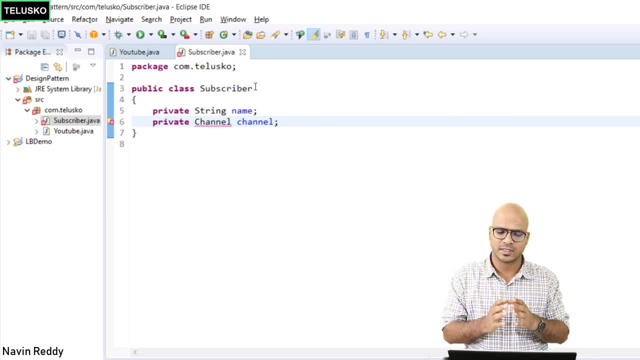 subscriber, that means you have subscribed a channel. See, I'm assuming that one subscriber will subscribe only one channel. now, I mean, one channel can have multiple subscribers, but one subscriber will have only one channel. But yes, on YouTube we have, we have this. 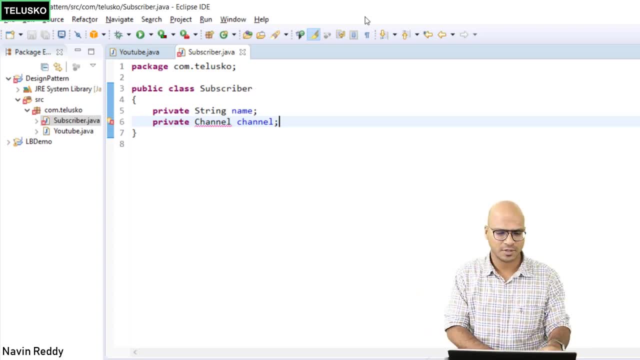 cross thing. Multiple subscribers can have multiple channels subscribed. But yeah, so let's. let's do this. So we have a string, name and channel, But unfortunately we don't have a class for this channel as of now, So let's create another class. I will say: click on that, create a channel. 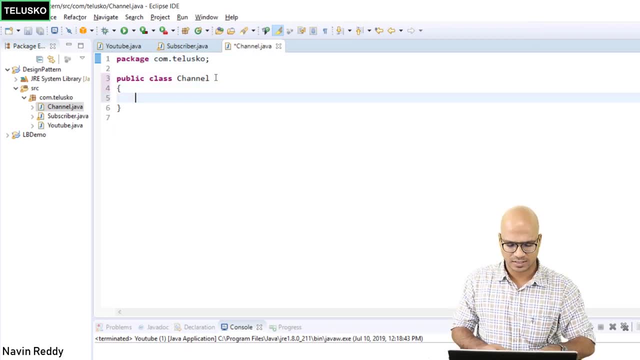 Yeah, so let's use the same package, which is comtodisco. So we got channel class. we will not be using this class as of now. let's only focus on subscriber. Now, when you say you're a subscriber, of course you want to know when I'm going to upload a new video. 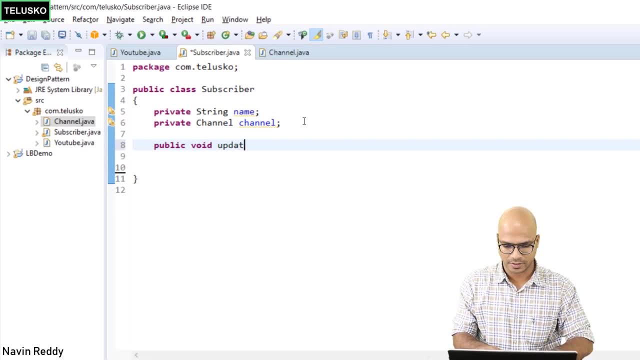 And the way you will get to know that is by using a method which is update. So let's say I'm going to upload a new video. So what this channel will do is every time I upload a video it will call this update method for all the subscribers. So let's say we have 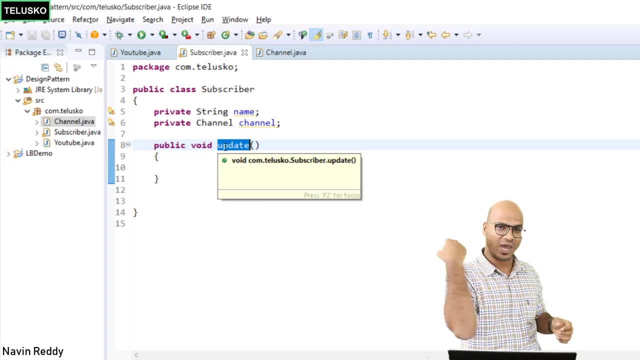 10 subscribers here, And then, the moment I upload a video, I will inform everyone. I will call all the update method of your objects, Right? So yeah, so that's the update method, And then in update, we can simply print a video uploaded. That's it, Nothing fancy. 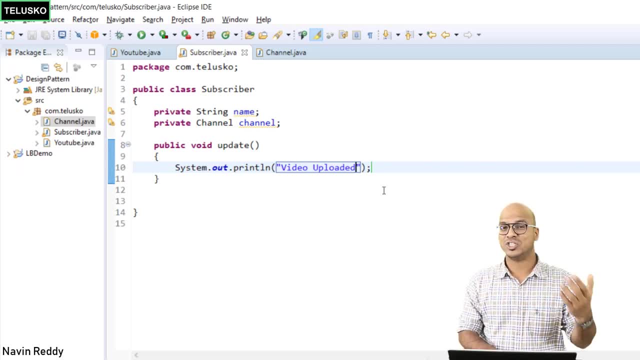 We're just saying we uploaded. I mean it should have said the title as well, And then which channel. but we are focusing on one channel, So let's ignore that. But let's say title: we'll do that in some time, And that's it. So that's one thing. And then we have to do: 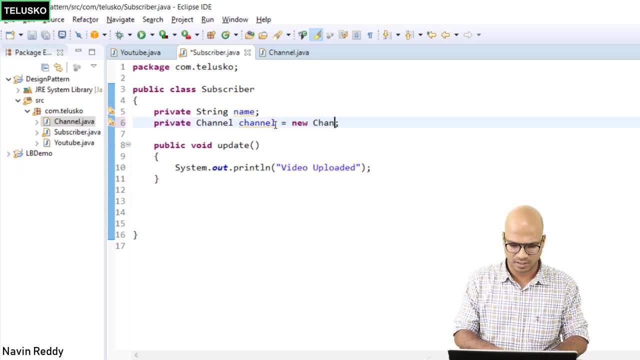 one more thing. First of all, we have to create the object for it. We'll say new channel. but that's a class, right, It should, it should have the object. But then what if you want to specify, or let's do that later. So yeah, so that's a subscriber Again. this is not. 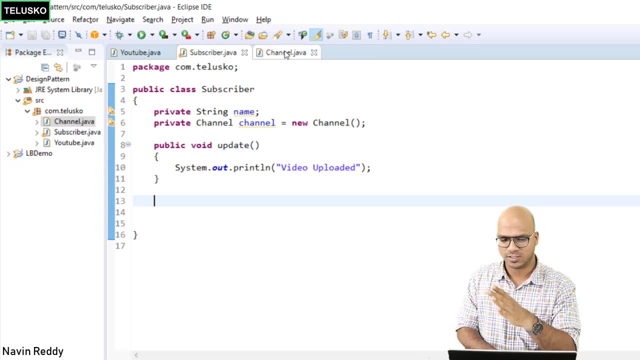 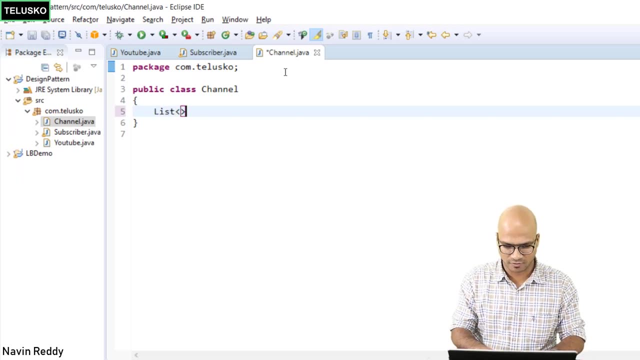 complete code. we'll do some modification there. Now let's move to channel. So what should be there in the channel Now? first of all, the channel should know how many subscribers it has. So here I will create a list of subscribers, I will say subs equal to, and then I will say: 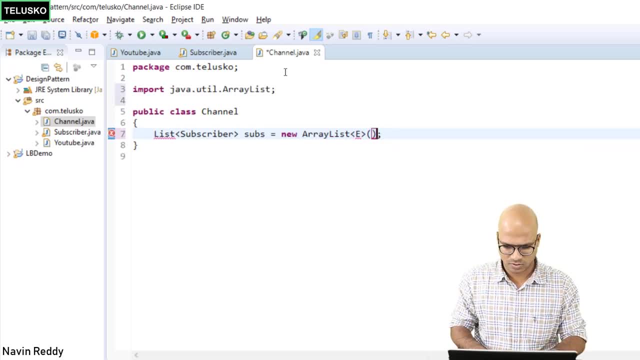 the new at least. So I want to create the blank subscribers. Yeah, let's import the package, for least. that's done. So you can see we got a list of subscribers Now. that's done Now. the next thing we need is: every time I upload a video, it should have a title as well. So I will say private. 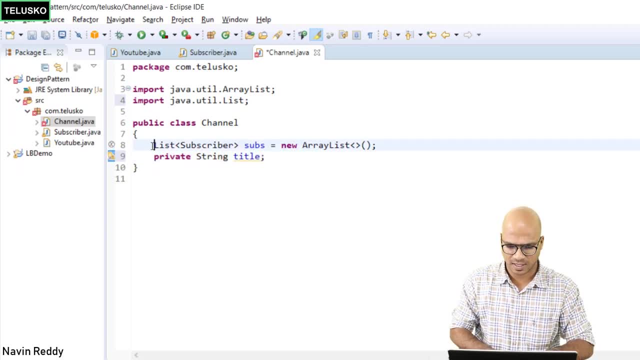 string title. In fact, I want to make this variable as private as well, the subs. Okay, that's done. Now in this we need some specific methods. The first one is register, unregister and update, or notify, you can say So. basically, we need a register, unregister and update. 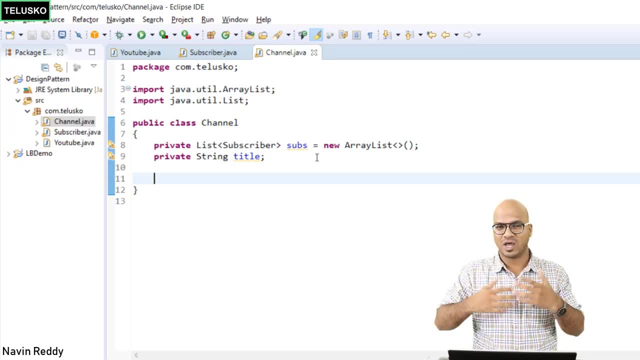 Now, what is register? So let's say, when I, when I started this channel, I was having no subscriber. I mean zero subscribers- Every time you subscribe to our channel so we get a new counter right. But we got new subscriber, So every day it is improving. Now you have 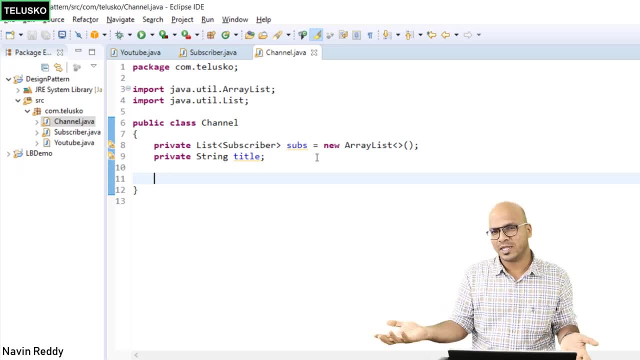 to. you have to register right And basically you have to subscribe. maybe some people unsubscribe, So let's say they don't, they don't want to follow the channel anymore, So they can unsubscribe. So we have these two options: subscribe and unsubscribe. We don't want to block you by 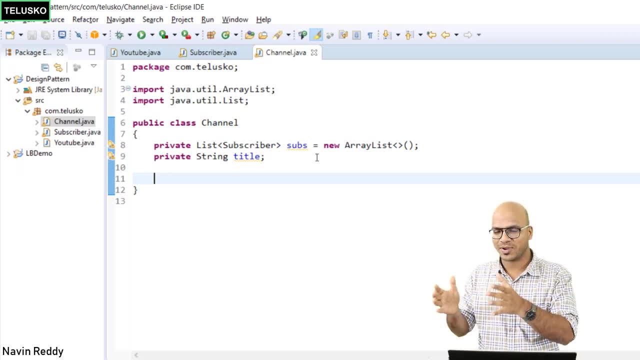 saying: hey, you can't unsubscribe, But yeah, so we can. we have subscribe and we have unsubscribe- two methods. So we just notify. the moment I upload a video, we will call notify method. Okay, so let's do that. So we'll say public void subscribe, that's the method And then in this subscribe, 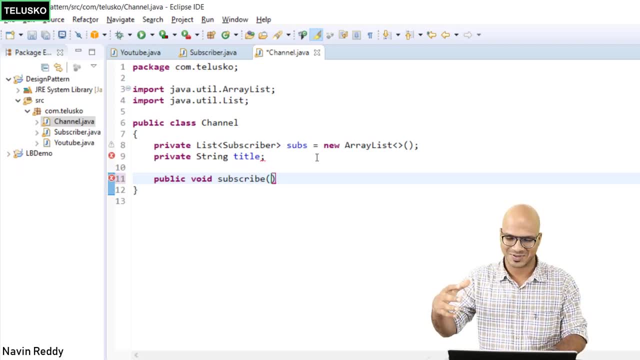 we have to mention which subscriber is subscribing. Okay, so we have somebody subscribed there. Okay, that's fine. So we have to mention the subscriber name here. subscribers sub. So every time you subscribe to our channel, we will get your object, the subscriber object. 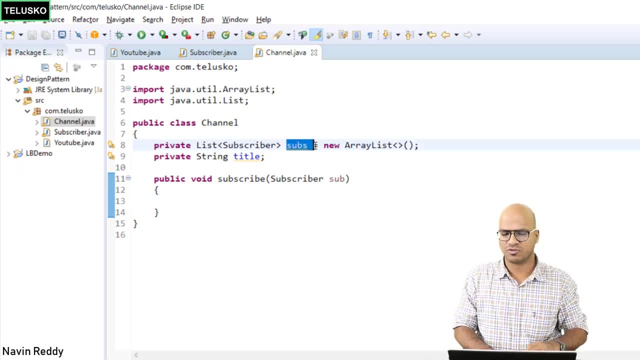 And then we just have to add that in this list. Maybe initially this list will be empty- 00 subscribers- But every time you subscribe it will add the new subscriber in the list. And the way you can do that, you can say subadd, And that's how you add the subscriber. simple stuff, right. 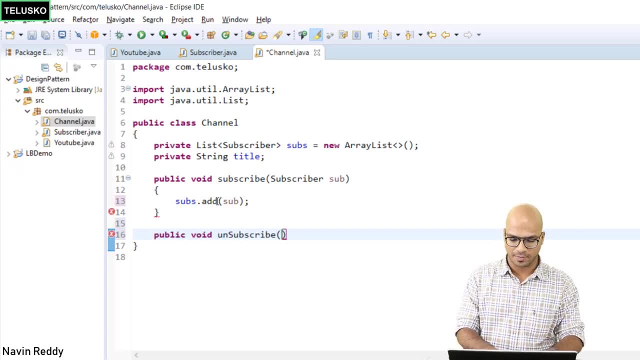 Now I want to unsubscribe in that case. So you will say public void unsubscribe. And here you will be having subscribers sub. Of course, right, when you unsubscribe you have to also mention which subscriber is unsubscribing. So we'll say sub Anyway. so I will say sub. 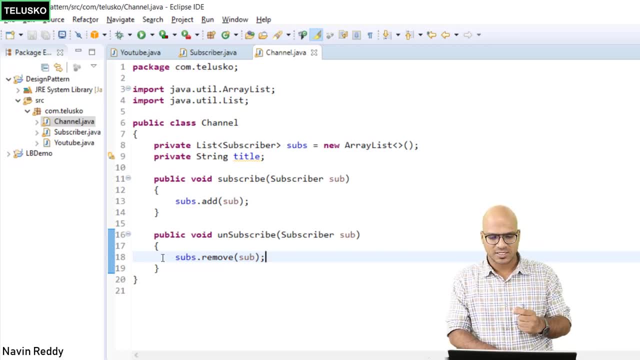 So we have, we are adding subscriber and we are removing subscriber. right, That's done. Now we have to notify the subscribers. How many subscribers, All right. For example, if I upload a video, every one of you should receive a notification And the way you can. 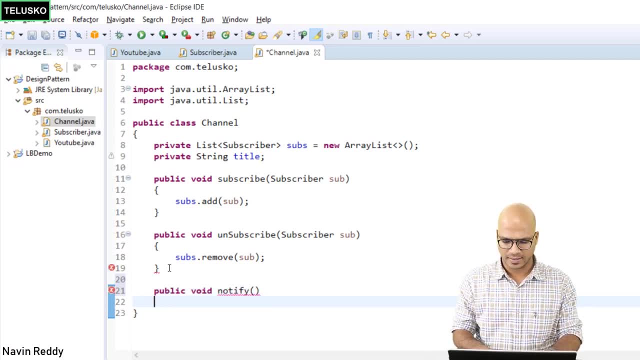 do that is by saying public void notified And then in this notify, you will call all the subscribers and then you will say update, update, update. Okay, But YouTube is not doing that nowadays, right? So every time we upload a video, YouTube, 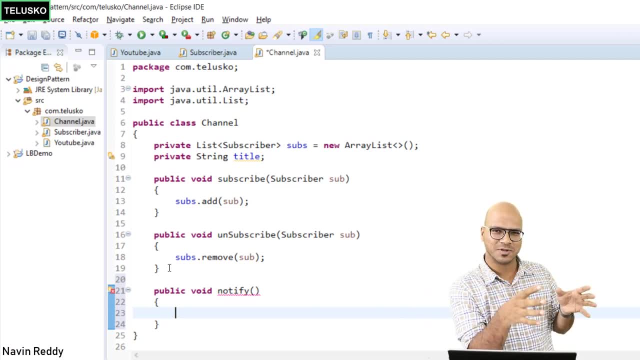 will not send notification to everyone. Maybe they will send 1000 people, And if those people are watching it, then they send to some subscribers, Right? But otherwise what we are going to do is we are going to change this. So in this case, we're going to change it to public void. 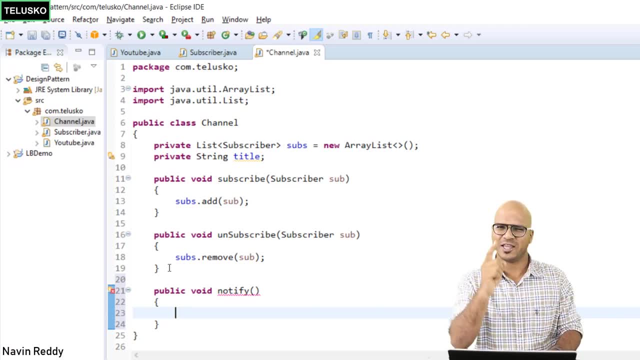 sent to some, some other subscribers, but we will not do that. we will inform everyone, and the way you can do that is you will use a for loop and then we can use normal for loop or you can use enhanced for loop. i hope you are comfortable with enhanced for loop. let's do that. so i will say: 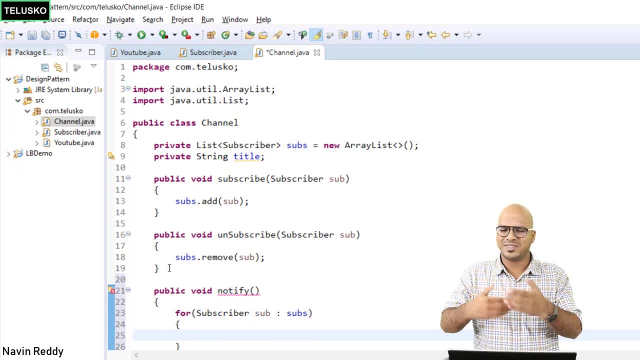 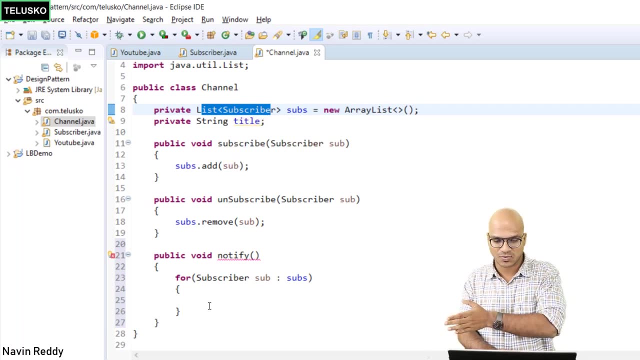 subscribers: sub colon subs. so we are basically iterating between all the subscribers in this list, right? let's say we have 10 subscribers, so we will be starting from the first subscriber to the last subscriber and then, in this for loop, you will be saying what you have to call the update. 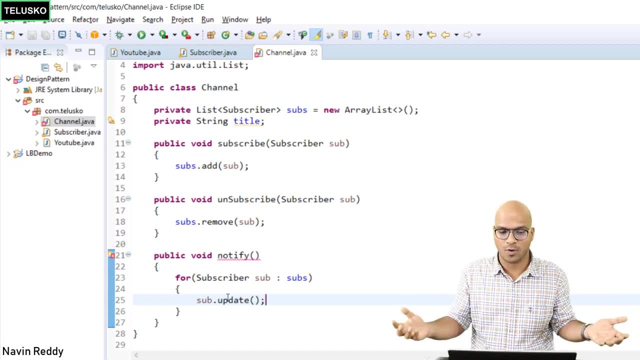 method. so basically you are calling update for each subscribers and then they will know: hey, video uploaded, right, so this works. oh, but we got an error here, okay. so basically we can't override this method because it notifies the inbuilt method, right. so i will say: notify subscribers. 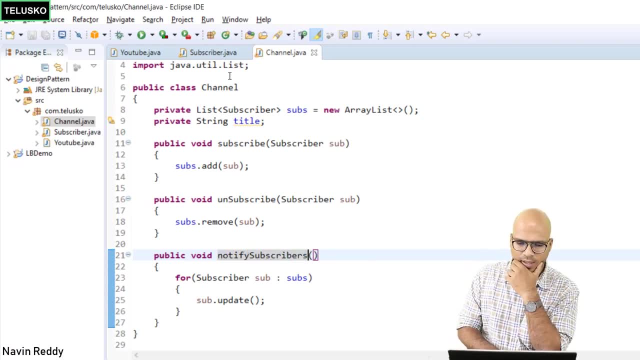 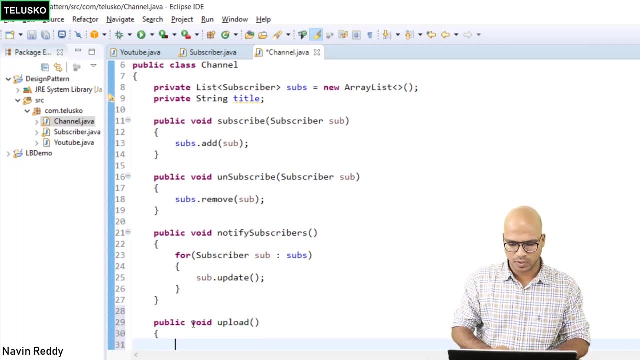 so you can see, we got these three methods, our job is done. okay, i will have one more method here, which is uploader. right, so every time i upload a video, so i will say public void upload, because in this upload i'm going to actually assign the title of the video. so i will say: 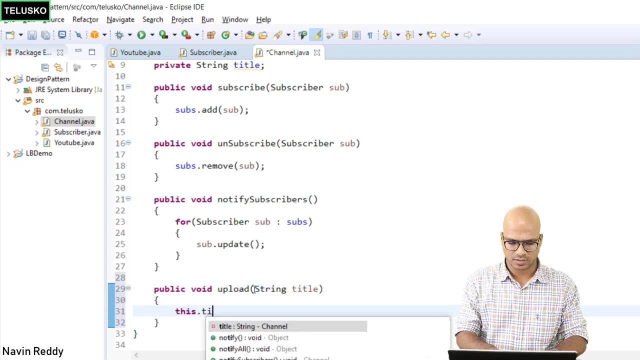 string title, and here i will say: this dot title is equal to title. and then. so who will call notify subscriber? is this here? so the moment i call upload a video, it will call notify subscriber automatically. so so that's done. so we got so many methods here and also we got subscribe, unsubscribe. 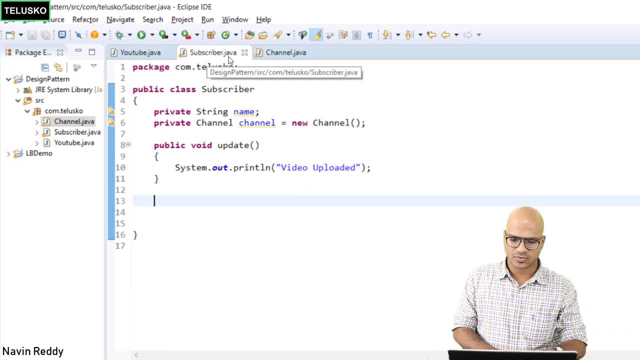 notify subscribers upload. and now i will go back to subscriber. do we need something more here? so a subscriber should know that we need something more here. so we need something more here. so we need which channel is subscribing? right? so we have to do that here as well. so i have to say public void. 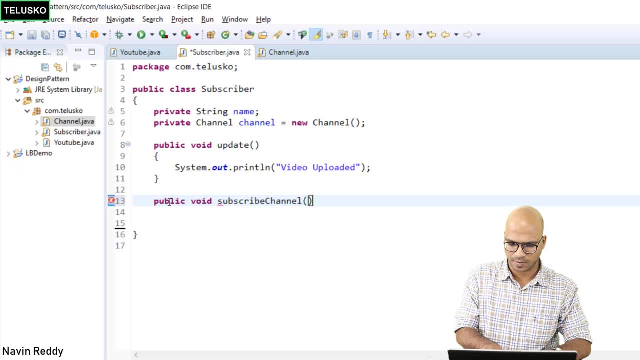 subscribe channel, because you need to know which channel you're subscribing. uh, so here you'll be having channel, maybe say ch and then you will say channel equal to ch. so basically, the moment you subscribe to a channel, it will update your channel name, so which channel you have subscribed, that's. 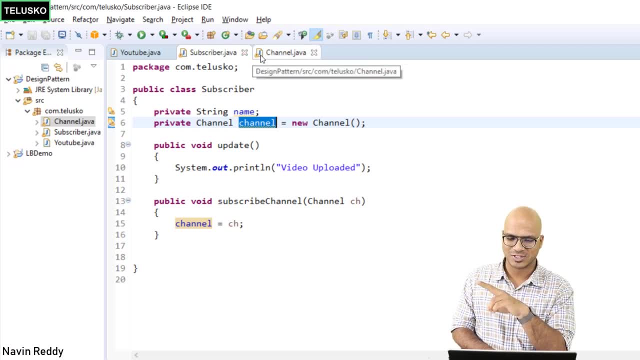 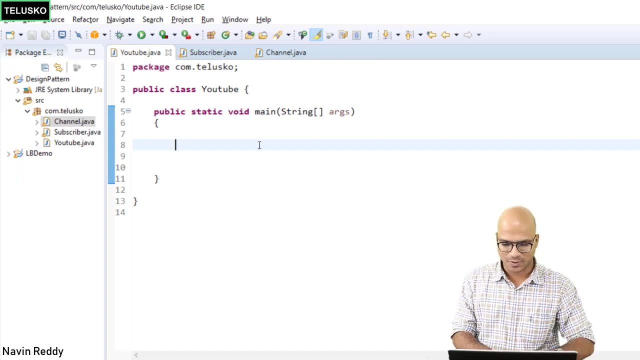 what it's saying. okay, so basically we got two class: one is subscriber, one is channel. i know it is going very lengthy, but it's it's quite simple actually. let's go to youtube and now let's perform the operation. so what i'll do is, first of all, i want to create channel. first i will say: 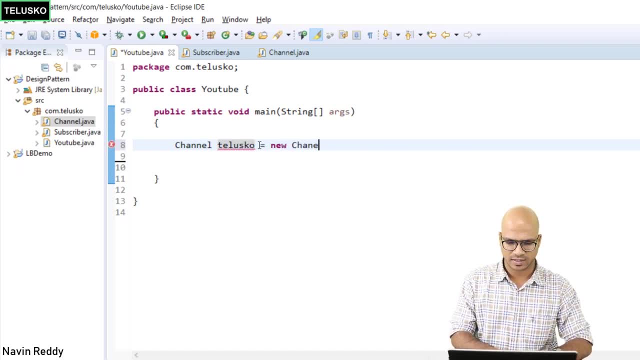 channel. the name is alisco. uh, equal to new channel. that's the channel we have. we can have multiple channels here, and then we want to create some new subscribers, right, so we'll have subscriber s1 equal to new subscriber. so we got this first subscriber, but then every subscriber needs a name. okay, i'm. 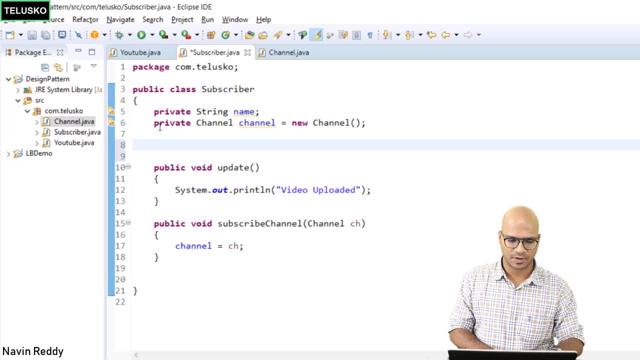 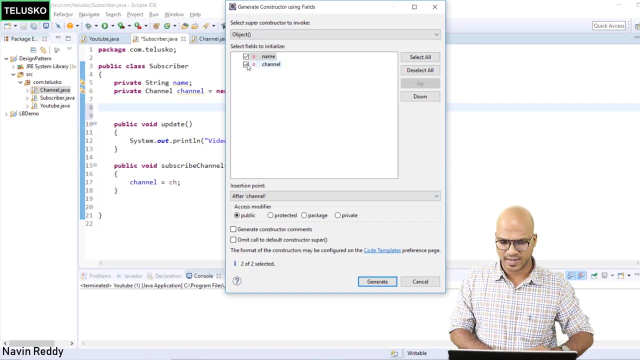 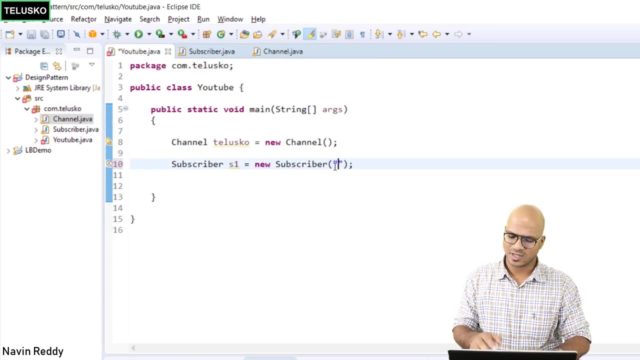 not doing that. so i will need a constructor from where i can pass the subscriber name. so i will say, right, like source, generate a constructor using fields, but not channel. i just need a name of the person, okay, so once you've got a subscriber constructor, let's go back here, and here we can mention a name. so that's the first. 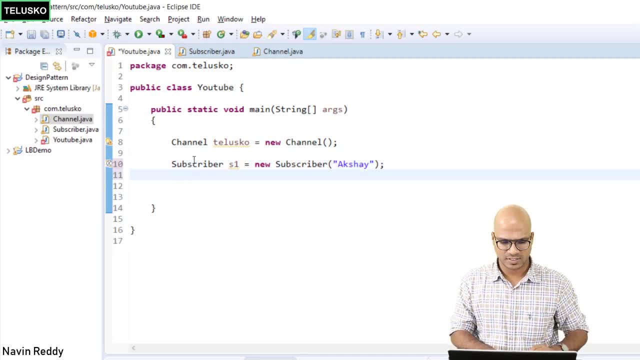 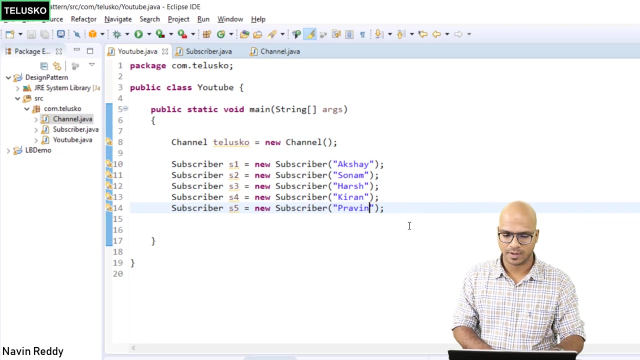 subscriber here is akshay, and then i will simply copy paste this. so say, copy, paste, paste, paste and paste. let's say we have five subscribers and the names would be, let's say sonam, say hush, so we got five subscribers here. so we have all these subscribers and their name. but now i want to add: 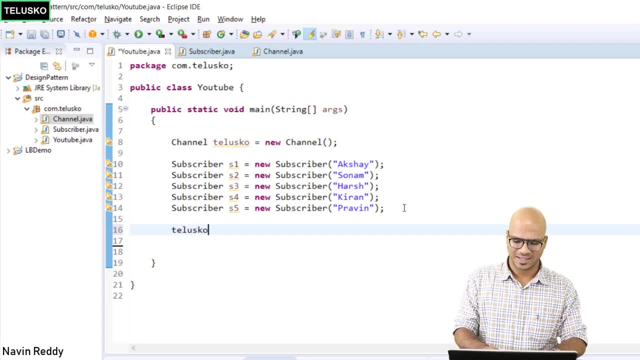 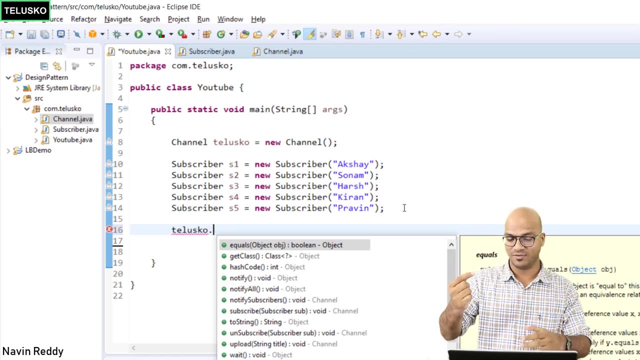 the subscriber to our channel, and the way you can do that is by saying: that is code dot. yes, you can also do that with gui. okay, so you can create a web application. uh, you can say subscribe and then it will add it based on your events. but since we are not doing that, we can have a. we can do that in. 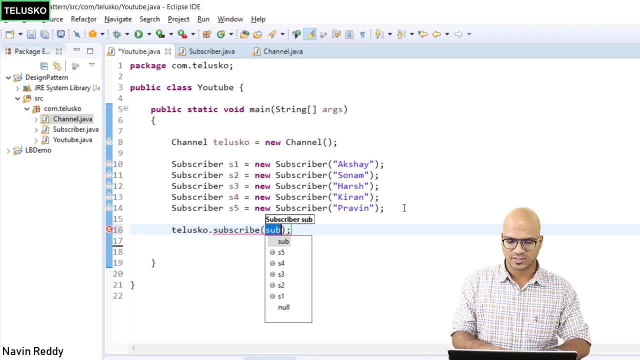 main method. so you can say: tele scott dot subscribe, so we are subscribed, the first user, which is s1, and then we can say the disco dot subscribe, which is s2, and then list goes on. i can simply copy this multiple times and let's update the values. okay, that's done. so terry's core has been subscribed. 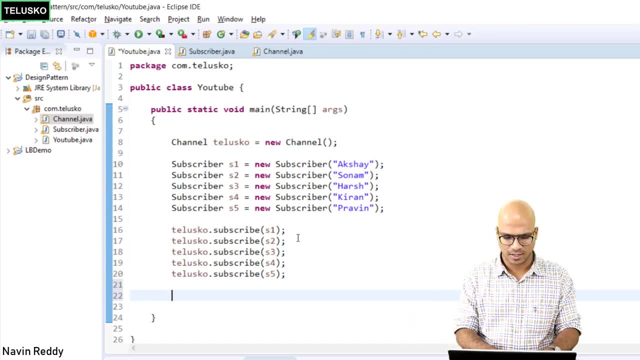 subscribers. in fact, even subscribers should know that which channel they have subscribed. so I will say s1 dot subscribe channel, because that's a event right. you will click on subscribe button, so we'll say subscribe channel, which is the risco. in fact, not just s1, every one will subscribe. so I will say copy paste. 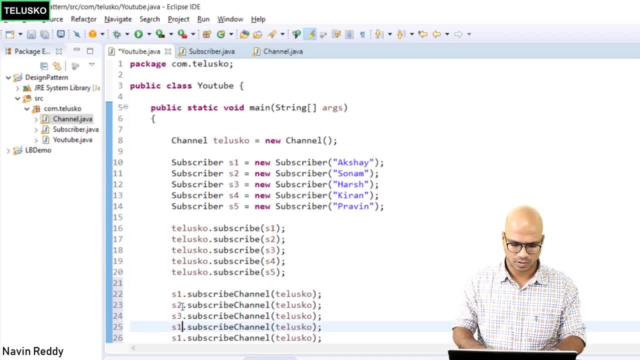 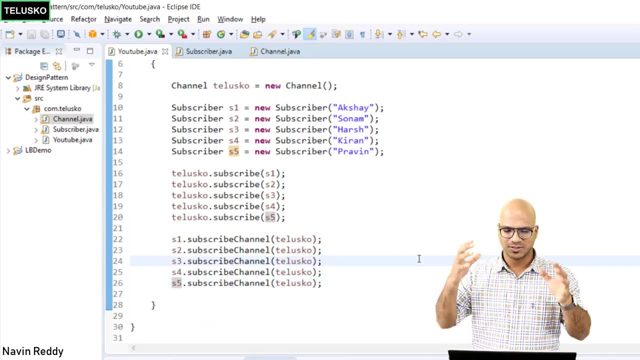 paste, paste, paste, and this will be two, three, four, five, and that's done. so. the risco knows their subscribers and subscribers knows which channel they have subscribed, and that's done. so basically, we got subscribers, we got channels, and then we are adding them. so now it's time to upload a new video. so I 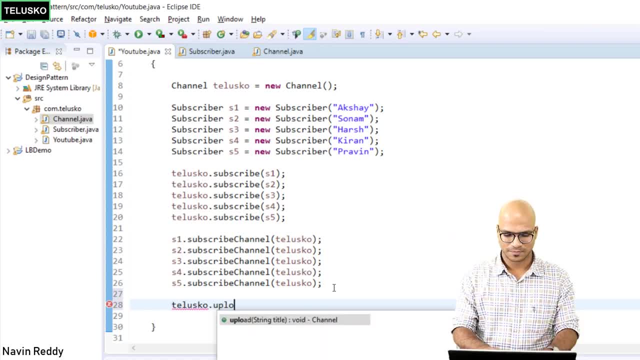 will say: the disco dot, let's upload a video. so we'll say: upload and I want to upload a new video which is I don't know. let's say how to learn programming. okay, so that's the video I'm uploading and now let's run this and let's see if that 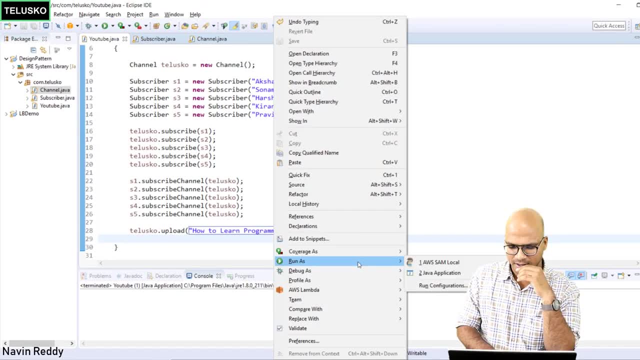 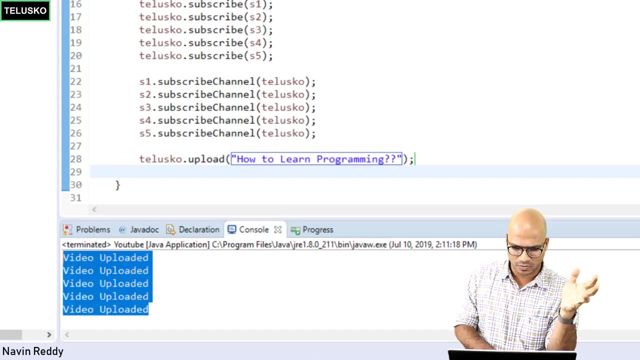 works, and if you get some error we'll solve that. let's right-click and say run as Java application. oh, it worked. can you see that every subscriber got the notification? but we don't know which subscriber got notification. so instead of just printing video uploaded will print, hey, and then I just 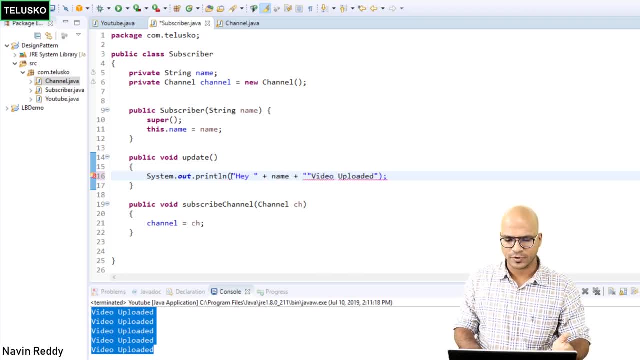 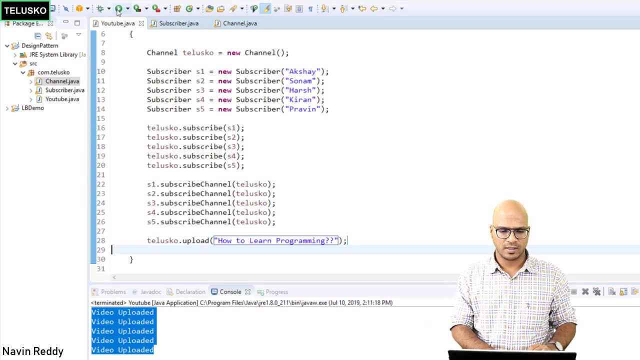 want to print their name plus. so basically, what it will do is it will say: hey, Naveen, video uploaded. hey, Kiran, video uploaded. that's what it will do. now let's run this once again and you can see it prints name and says video uploaded. of course there should be a comma, which I missed. yeah, so it will. 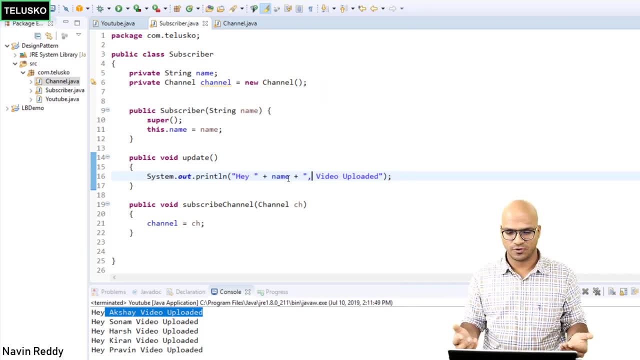 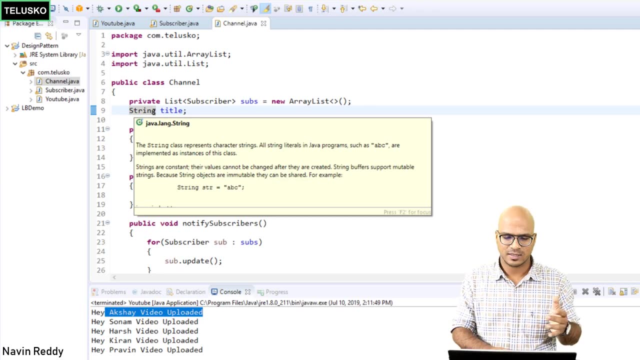 print. hey, Naveen video uploaded. but you can also print the title of a video if you want to. example, let's say, time win. I will not be making this as a private because I want to use it. use that in a separate class. that's not a good. 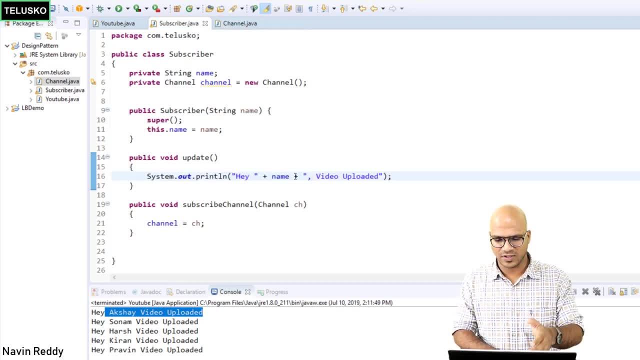 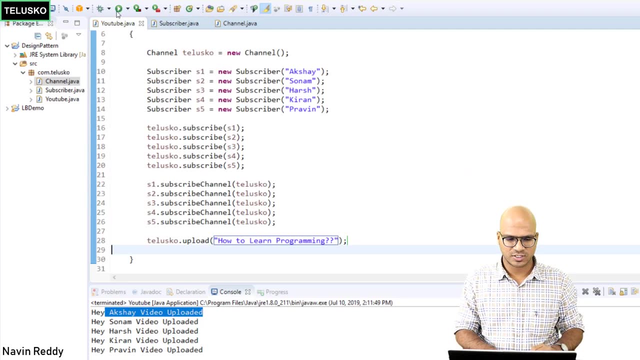 practice, but just to have less code, I'm doing that. so I will say: hey, Naveen, video uploaded and we also print the title here, which is channel dot title. so it will also be a title for you. and now let's run this and you can see it prints. 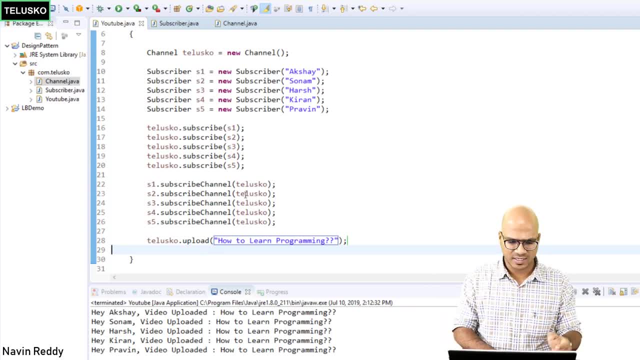 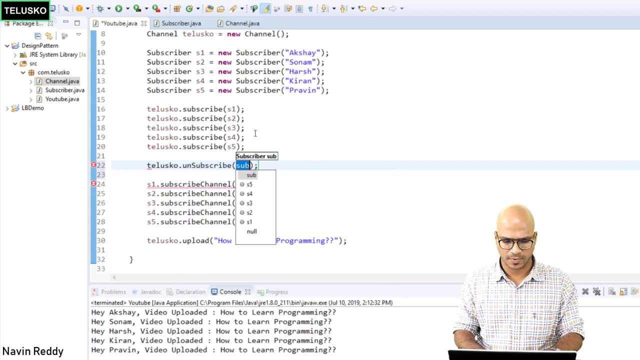 hey, Akshay video uploaded how to learn programming. but let's say, after some time someone says I want to unsubscribe. so let's say, after subscribing we are saying Tedisco dot unsubscribe. and who's unsubscribing? let's say s3, I don't know. who is s3 here? let's very quickly go ahead and say Tedisco dot unsubscribe and who's unsubscribing? let's say s3. I don't know who is s3 here. let's very quickly go ahead and say Tedisco dot unsubscribe and who's unsubscribing? let's say s3 here. let's say s3 is hush and let's say hush is. 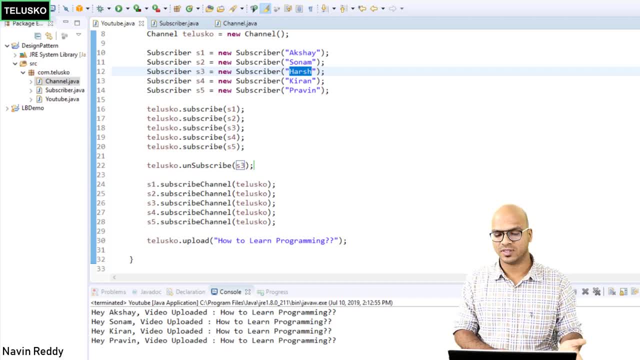 unsubscribe channel. and now, if you're on this, you can see hush is not receiving the notification now. so that's how this subscribe and unsubscribe thing works. so basically, all the subscribers here, they're observers. they're observing the subject, in this case a channel. every time we upload a video, they will get. 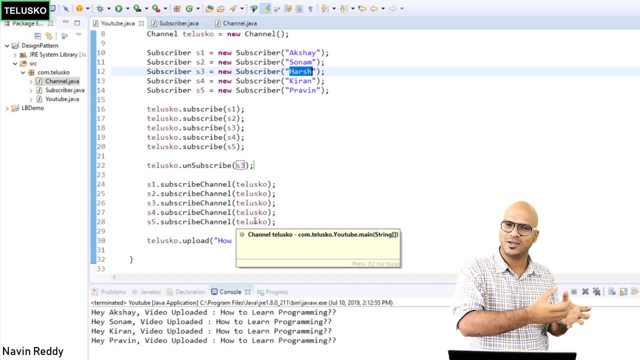 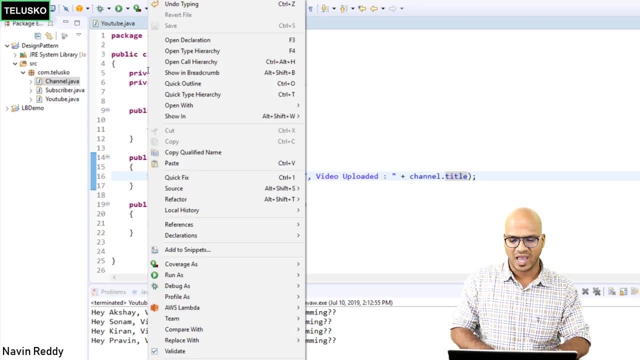 notification. it's more of a pushing from the subject to the observers. in fact, there's one more thing: when you implement this, all this is a concept of interfaces. so what I'm saying is the subscriber will be having its interface, will say: refactor, I want to create an interface out of it, and this interface 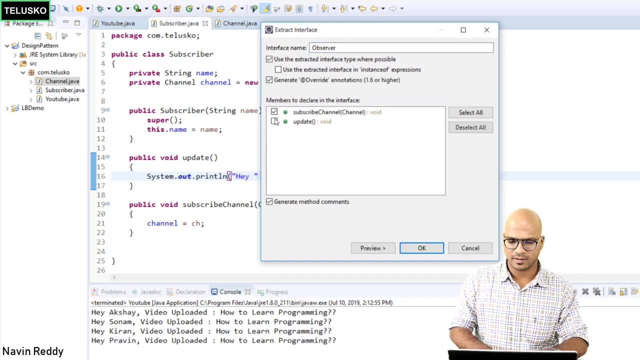 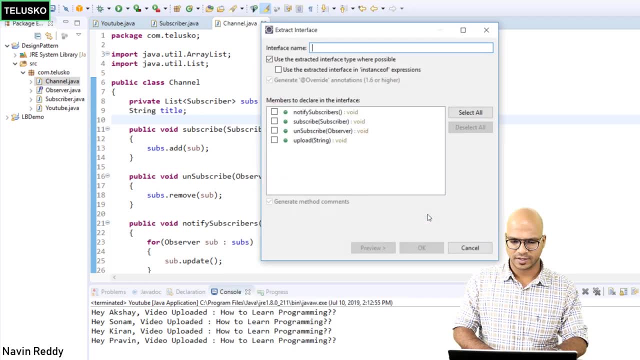 name would be observer, because subscribers are observer, and then it will have both the methods. so let's say observer, and now in channel as well, just do the same thing. I will say refactor, extract, interface, with all the methods, but name would be subject, right, so observer will observe the subject and 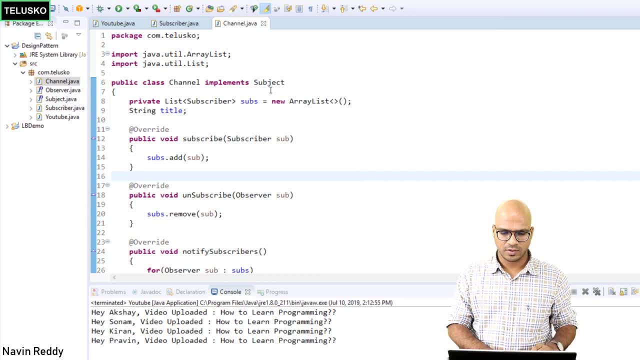 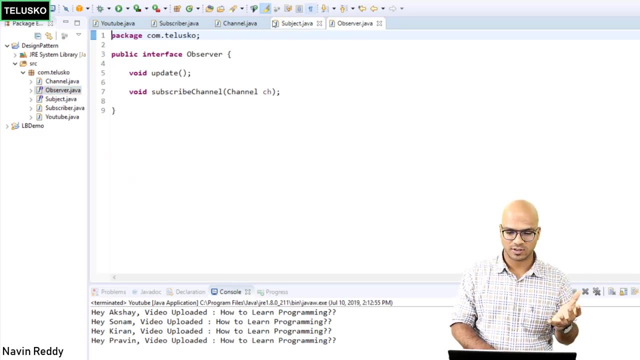 then even this will have all the methods. click on this and you can see we got channel implement. subject. and what is subject? it's a simple interface that have all the methods, simple interface with hash, which has all the methods, and in channel now you can see observer is getting subscribed. in fact, you can do that for this as well.